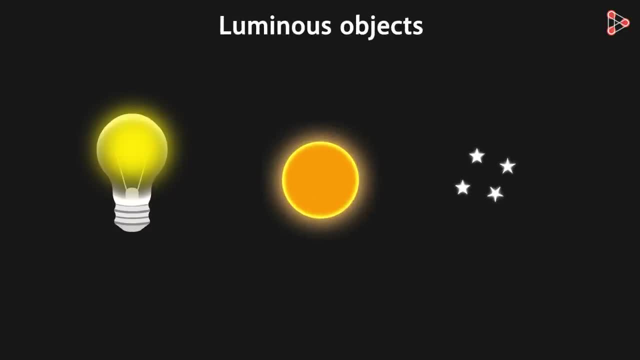 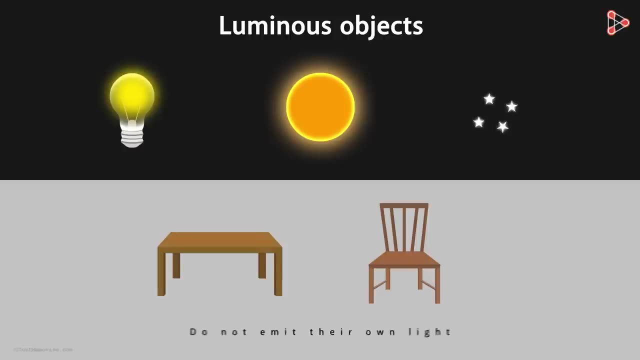 the stars are also luminous objects. What about objects such as this table and chair? Do they emit their own light? No, these objects do not emit their own light. Such objects are called non-luminous. Almost everything around us is luminous. 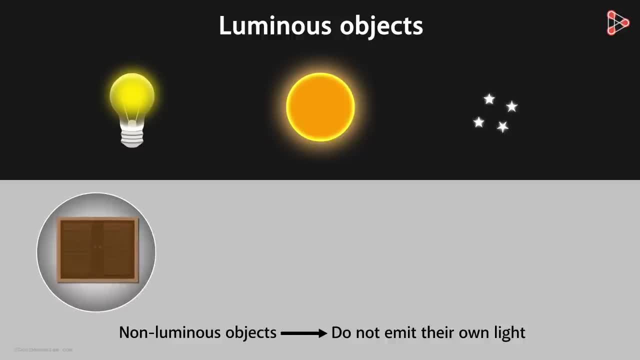 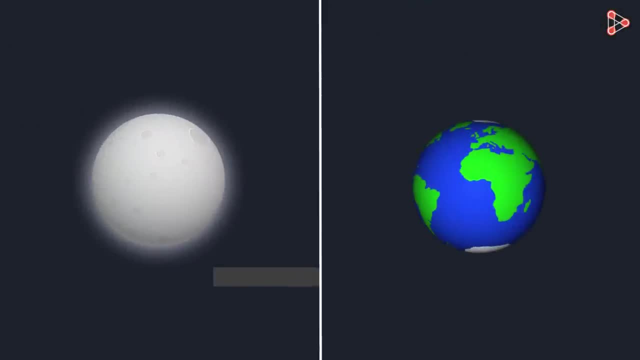 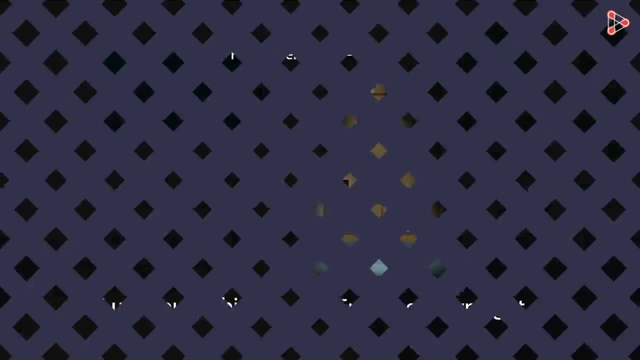 Objects made up of wood, plastic, cotton, metal are all non-luminous. What about the moon and the planets? They are also non-luminous. But if the moon is non-luminous, then how come we are able to see it at night? The answer to this is reflection. 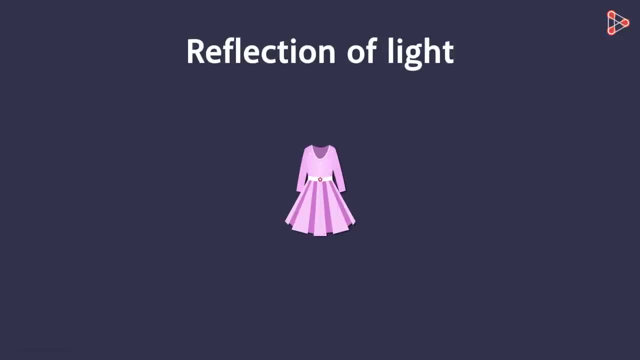 of light. The reason we are able to see any non-luminous objects around us is because of the reflection of light. Reflection of light can simply be referred to as change in direction of light or bouncing of light from some surface, Just like the ball bounces. 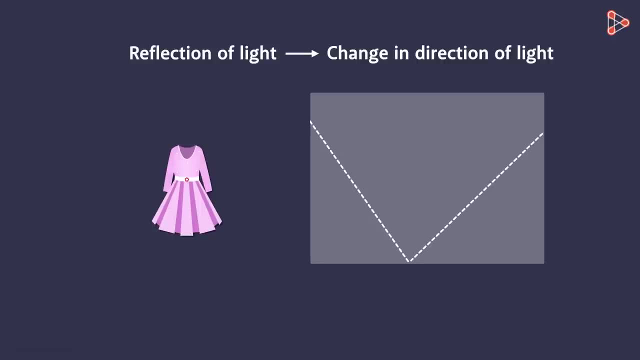 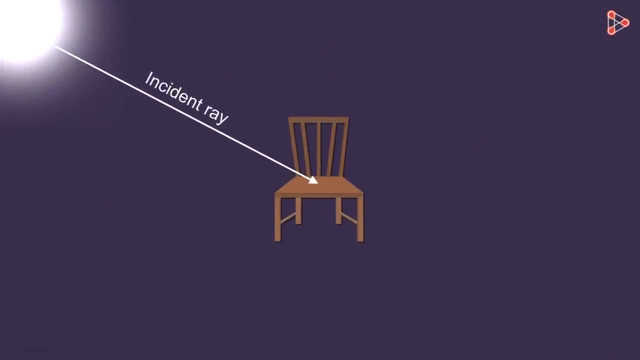 from the ground. light reflects off from a smooth surface. Let me try to explain it in a simple way. The light from the source strikes the object and bounces off from its surface, And when this light reaches our eyes, we see that object. 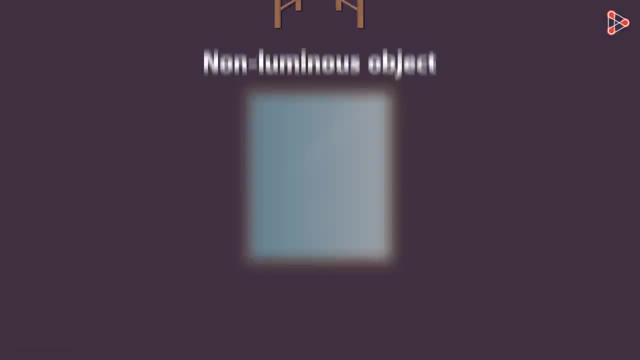 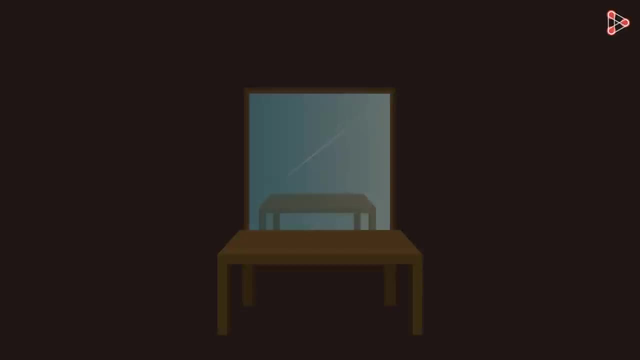 And this is how we see non-luminous objects. When the object is kept in front of the mirror, its image is totally very clear despite having lights, but when it is hit by a force, its image is formed in it. But will we be able to see the image in the dark? 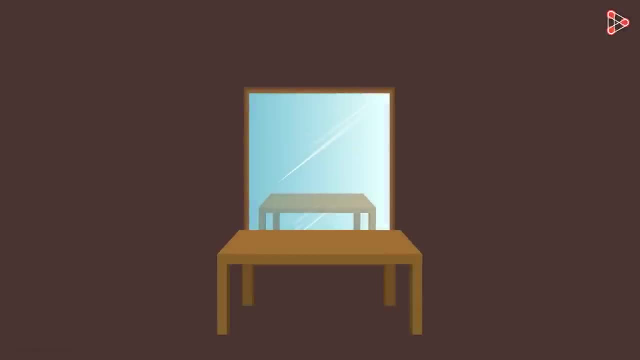 No, we won't. So the formation of the image is also due to reflection of light. Let this object be our human body. so, at the same time we are looking at the image, First tell me: is our body a luminous or a non-luminous object? 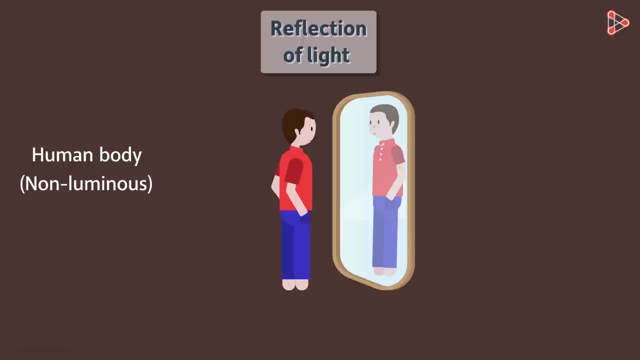 Well, it's non-luminous. Human body cannot emit its own light. So the light from the source is first incident on the human body. It gets reflected from it and this reflected light strikes the mirror. This light is further reflected from the surface of the mirror and reaches our eyes. 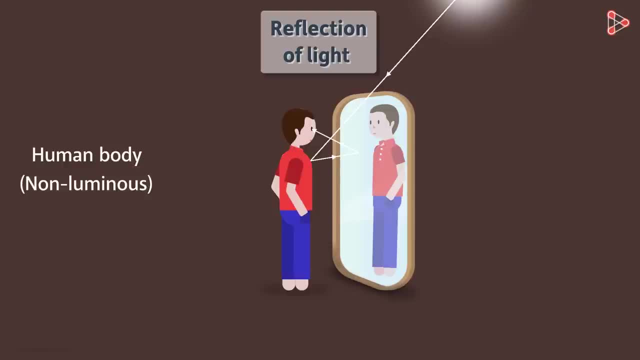 This is how we are able to see our image Now. obviously, this is not the exact picture of the happenings. I just wanted to give you the intuitive feeling into how this happens. There are a lot of subtleties involved, which we will learn. in our higher grades.